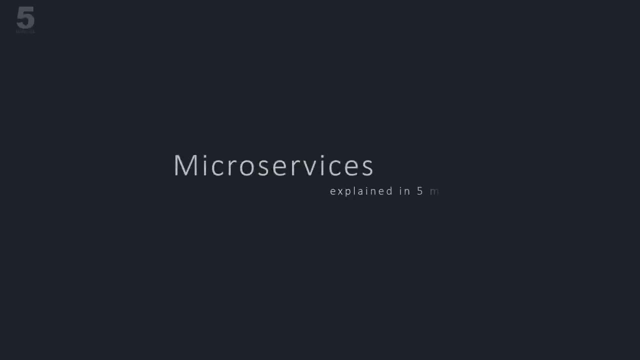 Microservices explained in five minutes. Microservices are a popular architectural paradigm that addresses the limitations and drawbacks of legacy applications. To understand the foundation of microservices, we need to take a look at the history and evolution of application design, from monolithic to multi-tier to microservice based architectures- A straightforward way. 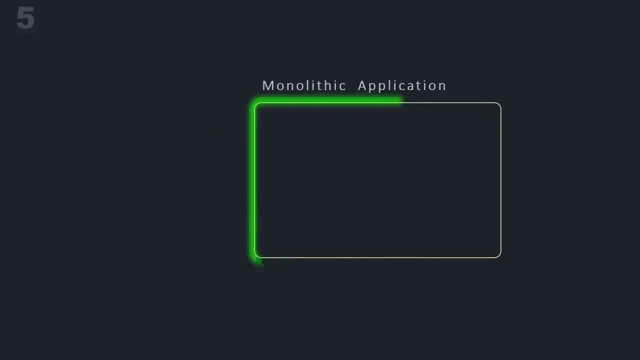 to build a simple application is to design it as a single piece of code encapsulating data storage and access, business logic and processes and user interfaces. That used to be the way applications and systems are designed and built in the early days Soon. 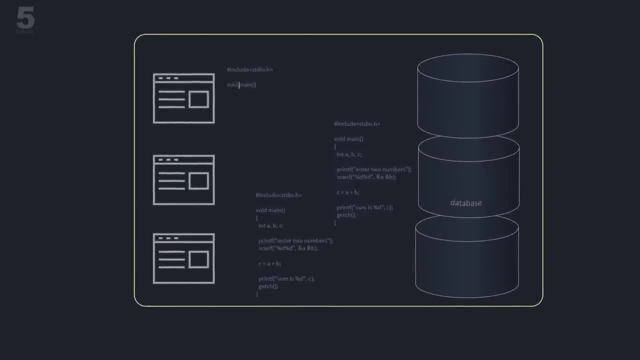 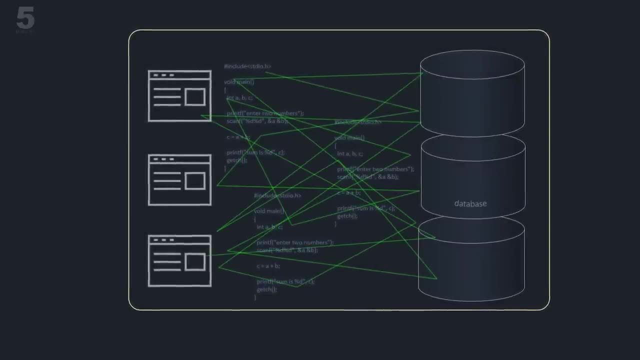 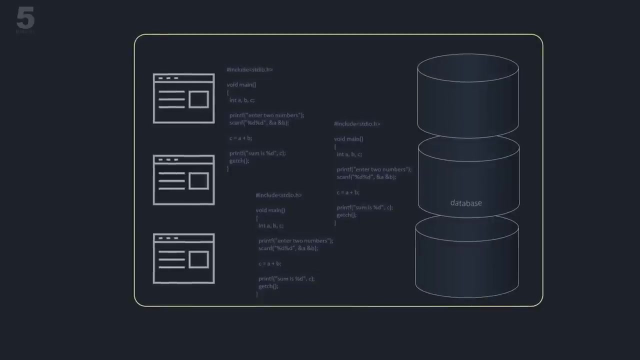 however, this all-in-one code model showed its limits when building complex, intricate systems. Since everything is tangled together, it becomes quickly difficult to maintain Software. engineers proposed a solution to this complexity problem: the multi-tier architecture, where application components are separated into layers based on technical functions. 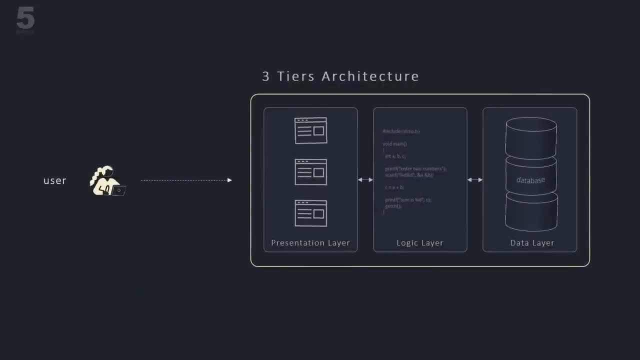 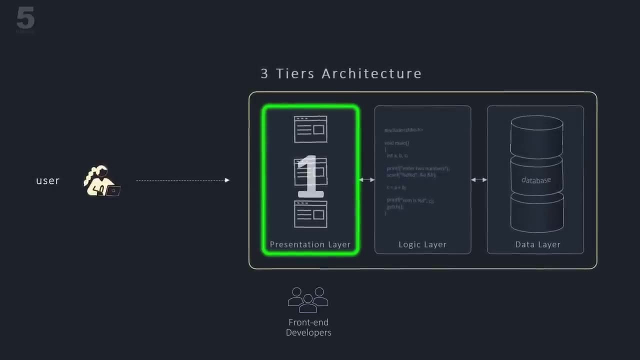 A common model is the three-tier architecture. It consists of three logical layers. A presentation layer covers all the code and components responsible for the interaction with users through visual interfaces. A logical layer encompasses the application components, which are the components that are responsible for the interaction with users through visual interfaces. A logical layer. 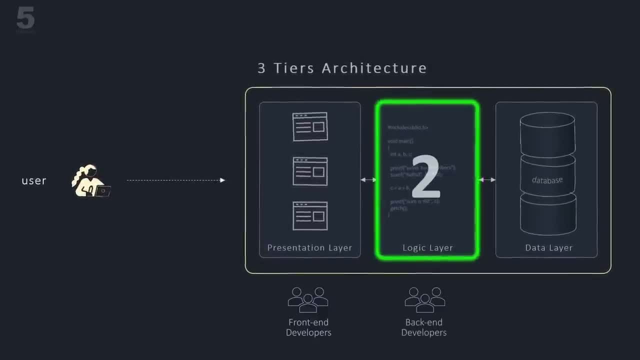 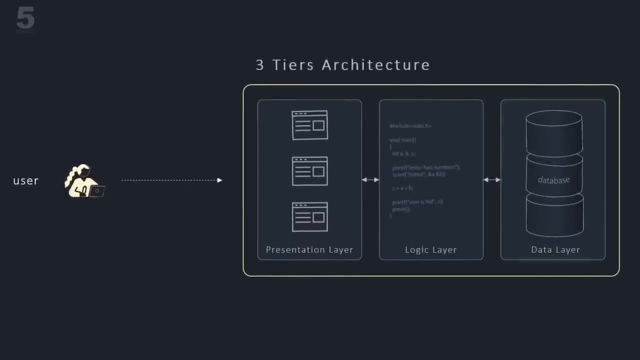 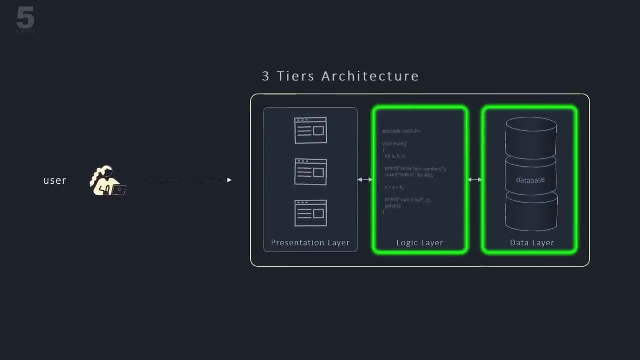 encompasses all the business logic and processes relative to the business functions And a data layer dealing with storing, accessing and retrieving data when needed. While separating logic and data in two different layers made things better, it was still a centralized way to designing an application and it didn't address quite well the challenges. 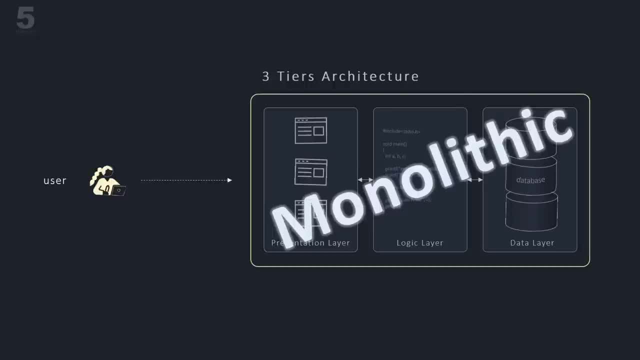 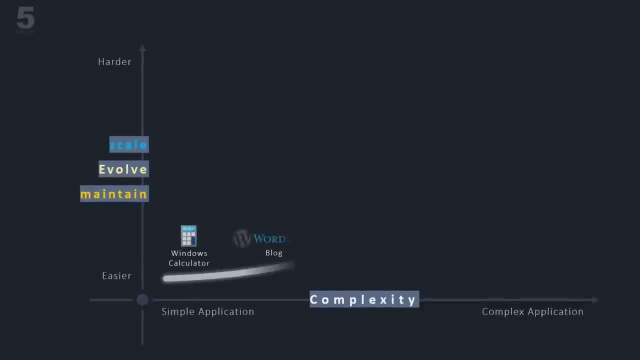 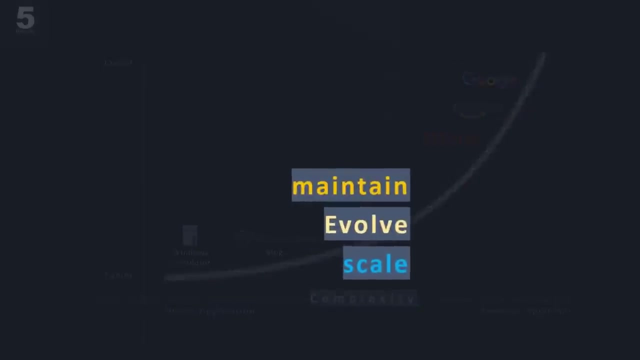 associated with complex applications and systems. Let's take a look at these challenges. Application complexity has been exponentially growing With the advent of global high-growth, fast-evolving web and mobile applications. maintaining evolving and scaling very complex applications like Amazon eCommerce website or Google search engine required a design. 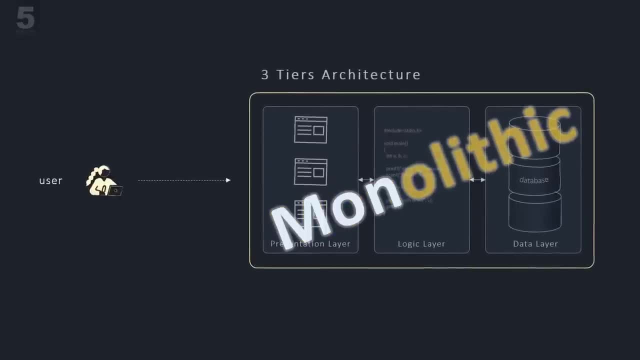 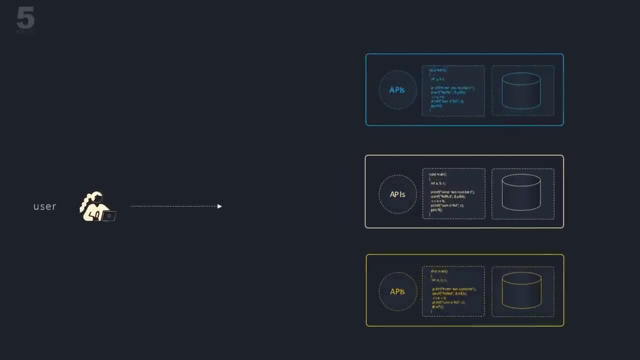 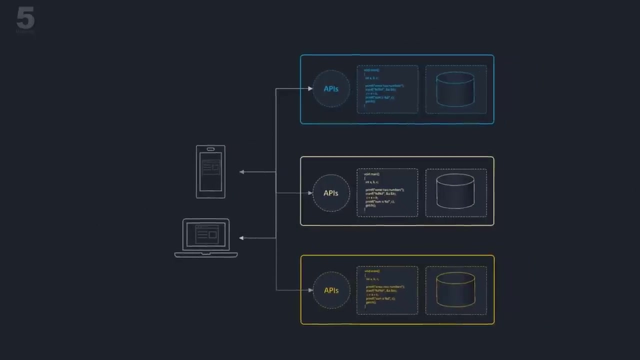 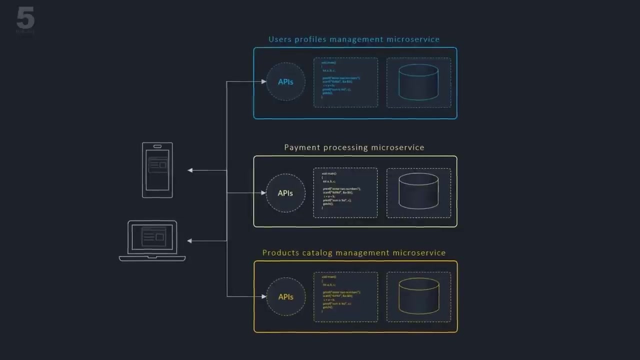 paradigm shift Here again. the best way to tackle complexity is by decomposing it into manageable chunks. That is why software engineers decided to break apart the logic and data layers into smaller pieces called microservices. Every microservice deals with one business function end-to-end, independently from other. 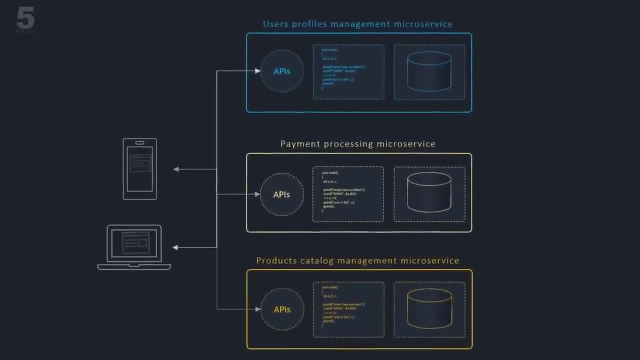 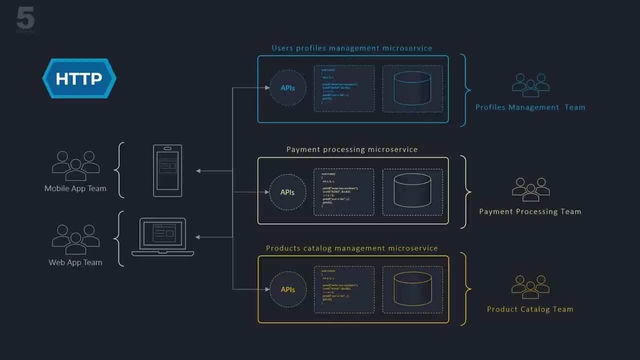 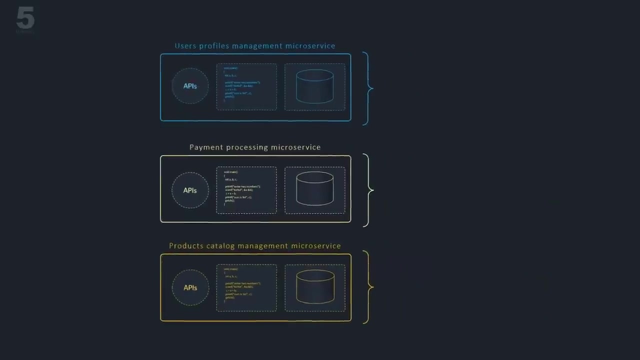 microservices. Microservices present simple, easy-to-understand APIs and communicate with each other through lightweight common protocols such as HTTP or message queues. When an application is architected, it needs to be designed in a way that allows it to work independently on different microservices. 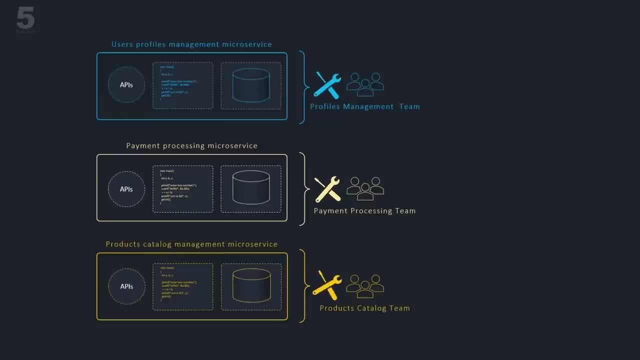 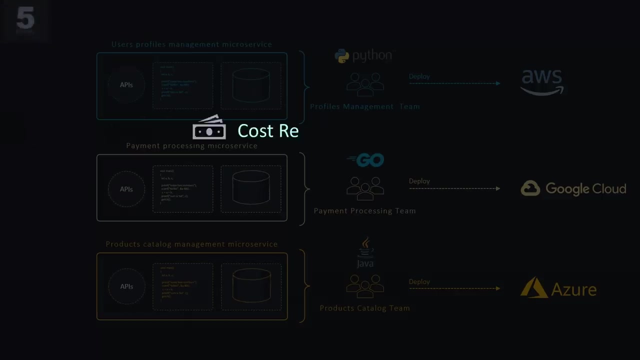 Building new functions and evolving the business capabilities without impacting other teams and business functions. Theoretically, teams could even use different programming languages and deploy their microservices to different infrastructure. However, for cost reduction, efficiency improvement and operational optimization needs it is. 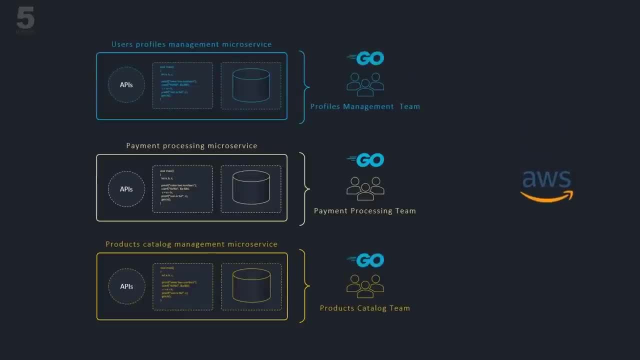 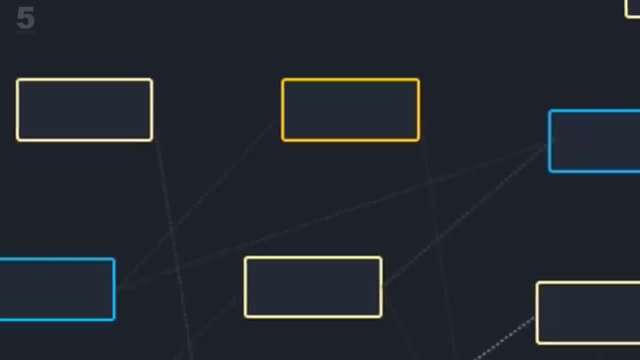 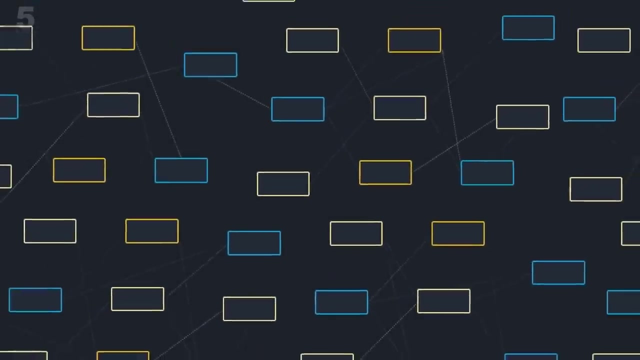 not possible. Most organizations limit team choices to a set of approved tools, infrastructure providers and programming languages. As applications continue evolving and growing, the number of microservices inside an organization could expand to tens, hundreds or even thousands. As this happens, complexity starts creeping again. 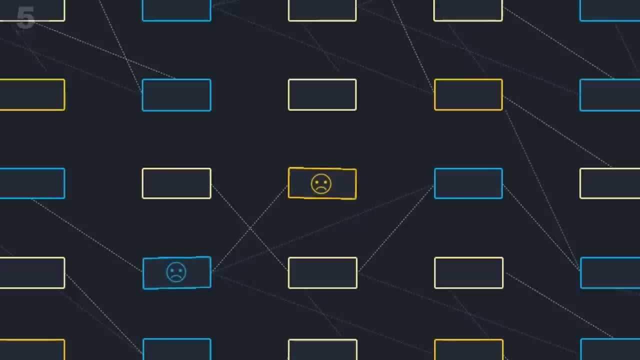 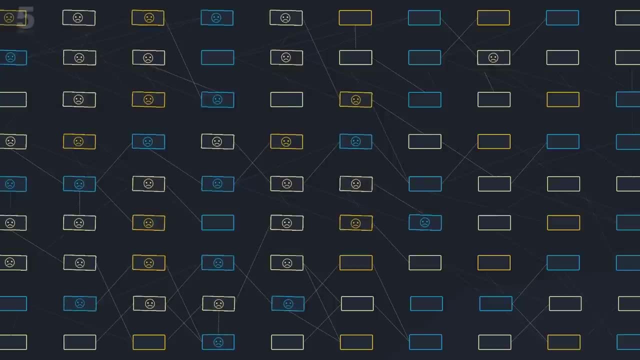 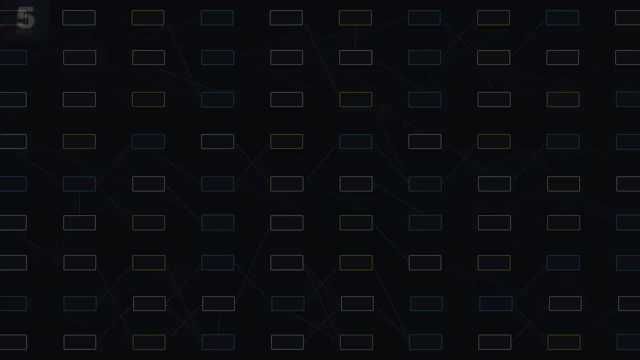 For example, if a microservice instance fails in production, it could generate a cascade of outages within other microservices. Since the architecture is highly distributed, it could become difficult to identify the root cause and fix it in a timely manner. The software engineering community has been creating and inventing new tools to tackle 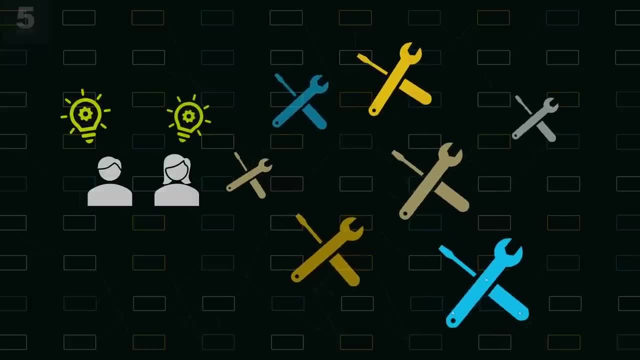 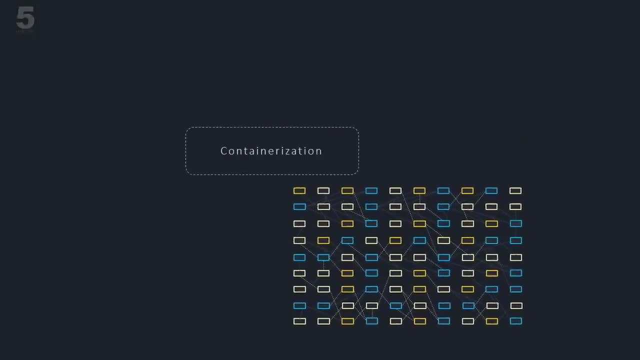 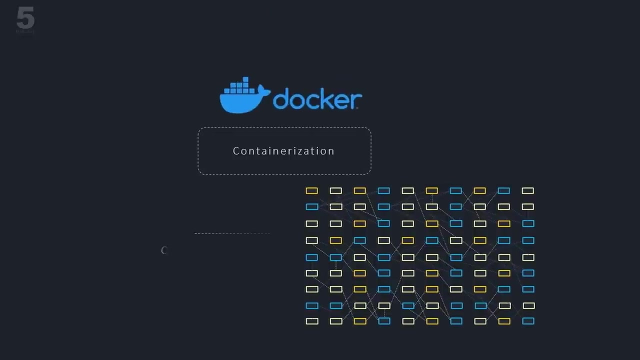 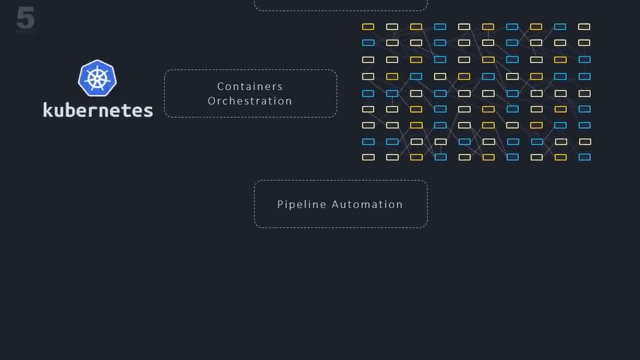 and contain the ever-growing complexity of highly distributed microservice-based systems. Some of the popular tools include: containerization that helps deploy microservices in minimalist, self-contained runtimes. Container orchestration systems that manage containers' life cycle, such as Kubernetes. Pipeline automation for CI-CD.